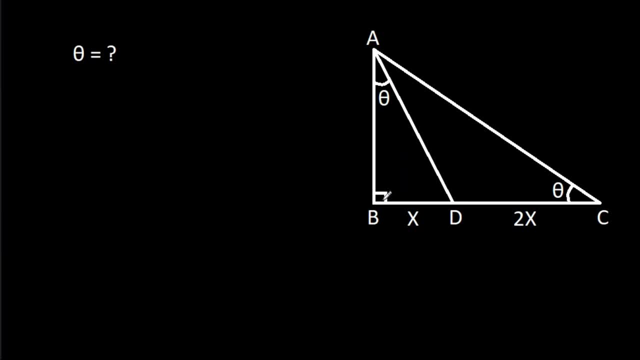 In this video we have been given a right angular angle, ABC, and angle BAD is theta, angle ACB is theta and BD is x, CD is 2x, Then we have to find theta. So the first method: if we extend DB to suppose E, then this angle it will be 90 degree And if we join AE. 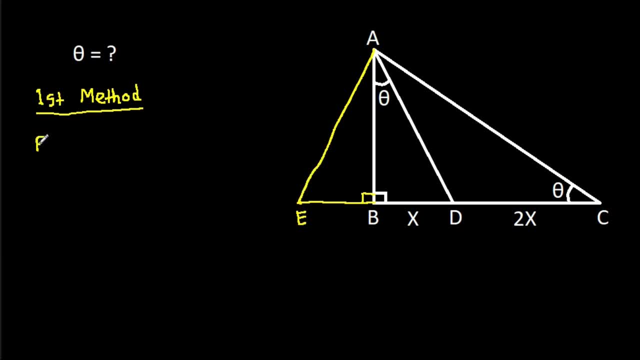 such that BD it is equal to BE. it is our construction. Then triangle BAE it will be congruent to triangle BAD Because we have BE is equal to BD and angle EBA it is equal to angle DBA. that is, 90 degree. 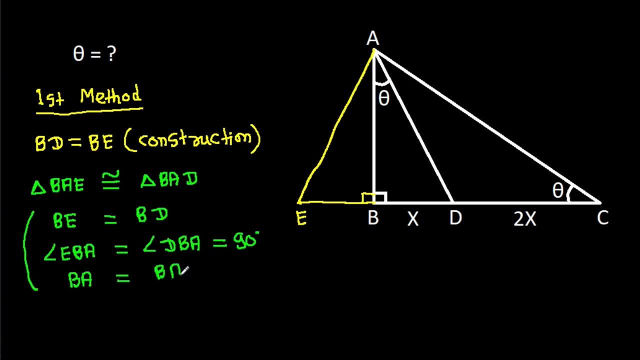 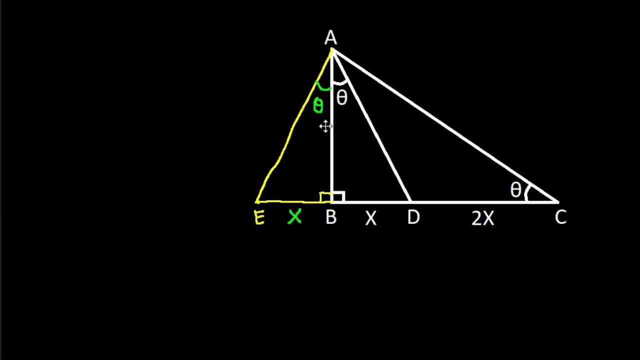 And BA is common, So angle BAe it will be equal to angle BAD, and angle BAD is theta, so this angle it will be also theta. and BD is x, so BAe, it will be also x. And now, now, now. 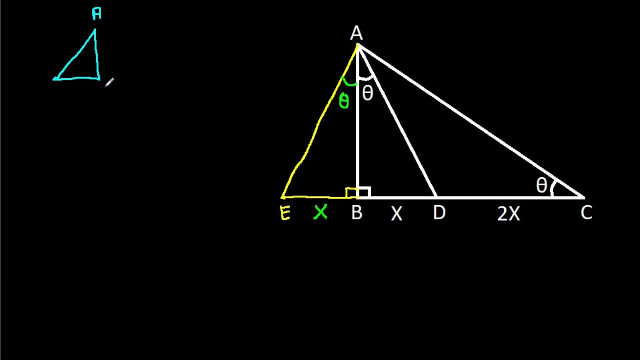 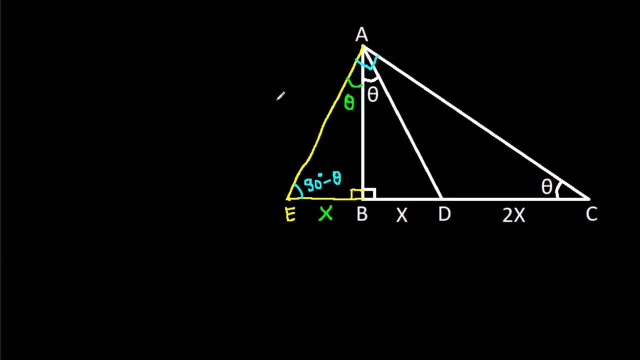 now, in any right-angled triangle, ABC, if we make a circle around ABC, then in in any circle diameter diameter makes an angle of 90 degree on the circle and we have angle BSC is 90 degree. that means BC. it will be diameter. so the 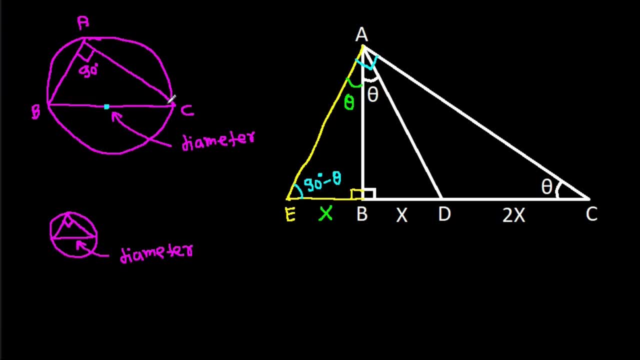 center of the circle it will be on BC. suppose O and OB, it will be equal to OC, that will be equal to OA, that will be radius of circle, and here from point D, we, that will be equal to D estructan. so they areенные two. 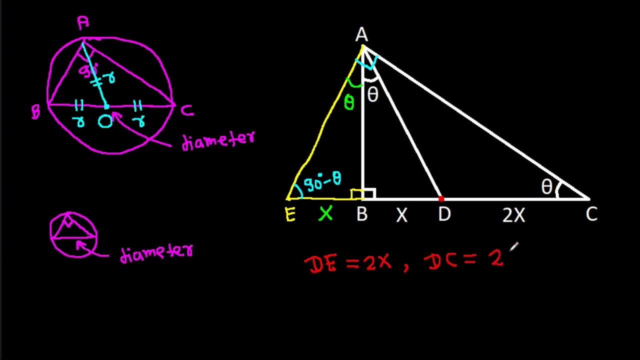 and these wanted in l, then this will be also 2x, so들이 both. so that means we hasล will use c, that means both are gonna be, or we have BE it 2x and DC is k. so wir haben BE, das ist 2x und das ist auch 2x, so dra will also 2x. 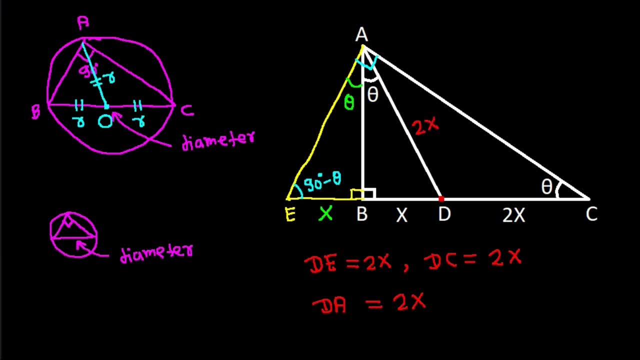 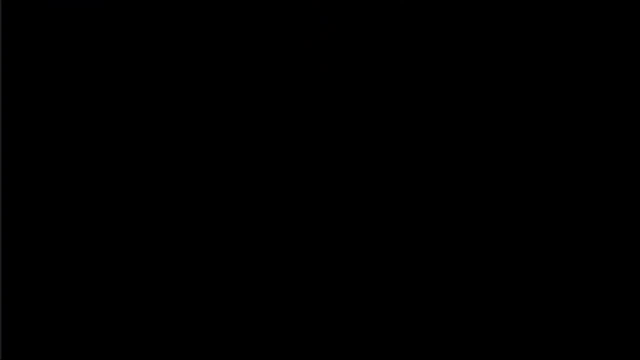 so da WILL also 2x, DA it WILL also 2x, 3x. and Now in triangle, ADC we have, AD is equal to CD, that is 2x. That means these two angles they will be equal And this angle is theta. so this angle it will be also theta. 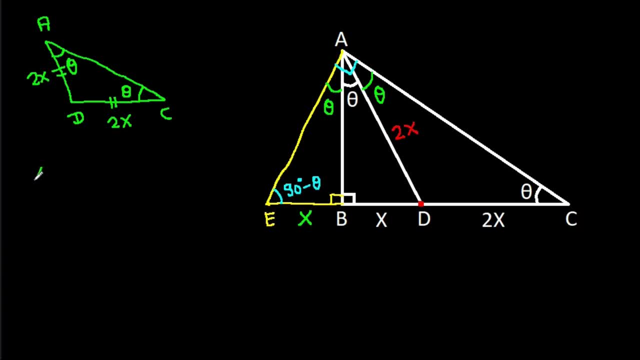 This angle it will be theta And we have angle ESC is 90 degree And angle ESC it is theta plus theta plus theta That is 90 degree And 3 theta it is 90 degree. So theta it will be 90 degree over 3, that will be 30 degree. 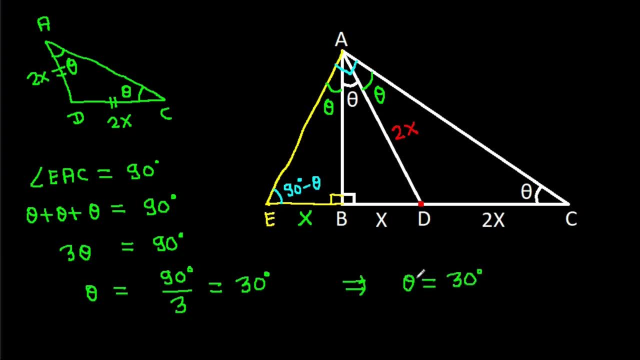 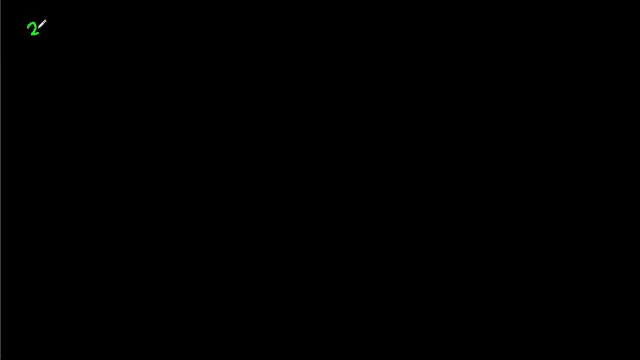 So we get: theta is 30 degree. And this second method: Okay, Inter angle, ABD, it is ABD, this angle is 90 degree. This angle is theta, So tan theta, it will be BD over AB, So this angle is 90 degree. 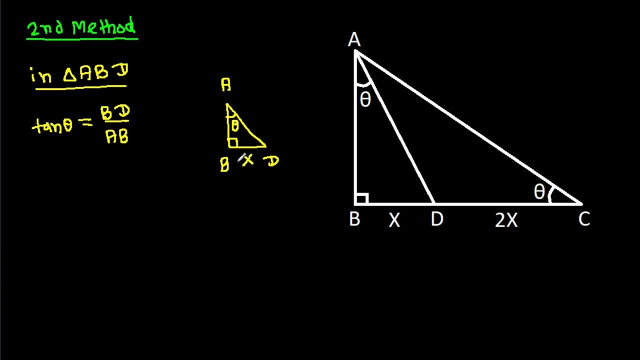 This angle is theta, So tan theta, it will be BD over AB And BD is x, So it is x over AB. And inter angle ABC. it is ABC. This angle is 90 degree. This angle is theta And BC it is x plus 2x. 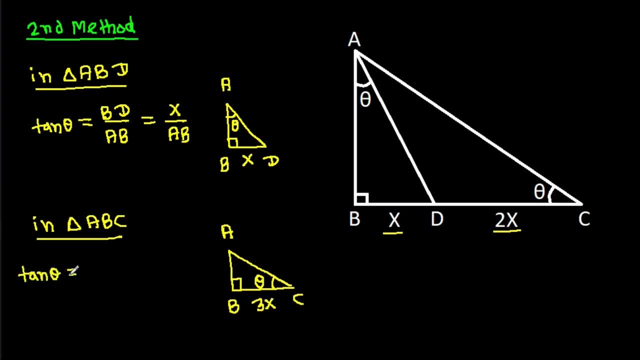 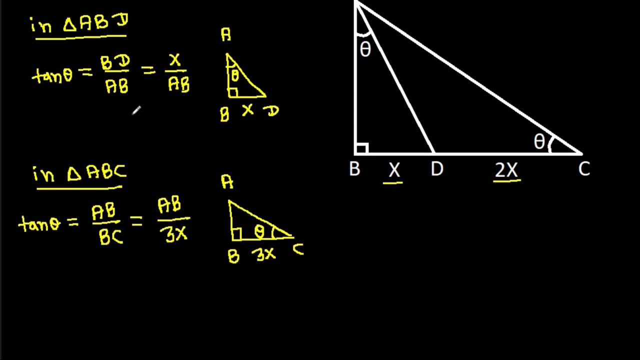 That will be 3x And tan theta it will be AB over BC And it is AB over BC is 3x. And from these two equations we have tan theta is x over AB And it is AB over 3x. 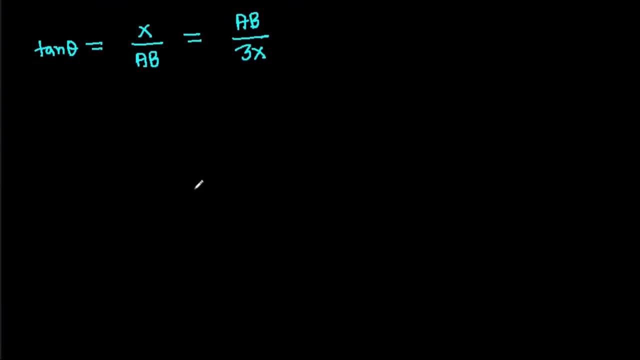 And we have x over AB, is AB over 3x And if we cross multiply, then 3x s square it will be AB s square, So AB it will be root under 3x s square, that will be root 3.. 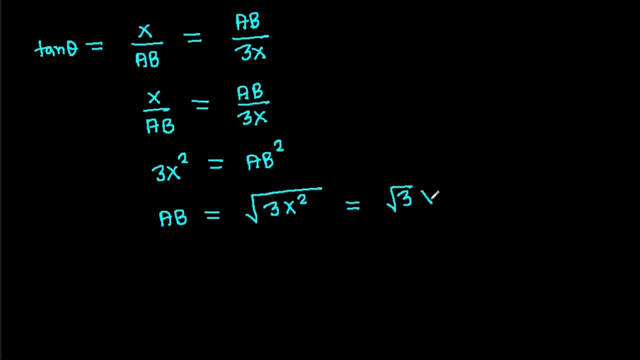 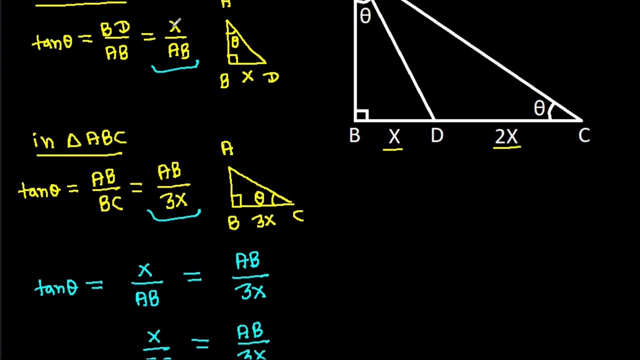 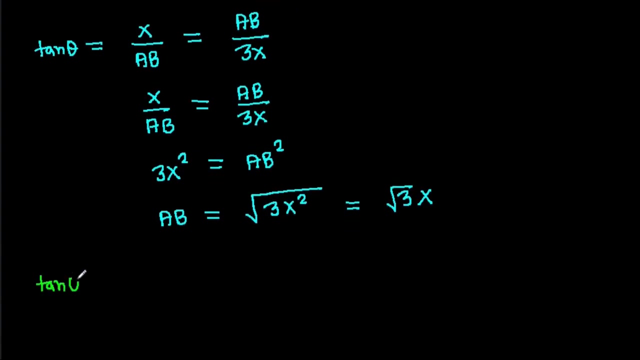 Then x over AB is 3x, Then 3x is a square, Then x over 3x is a square, Then 3x is a square, x and we have tan theta is x over a b. We have tan theta is x over a, b and it is x over a, b is root 3 x. 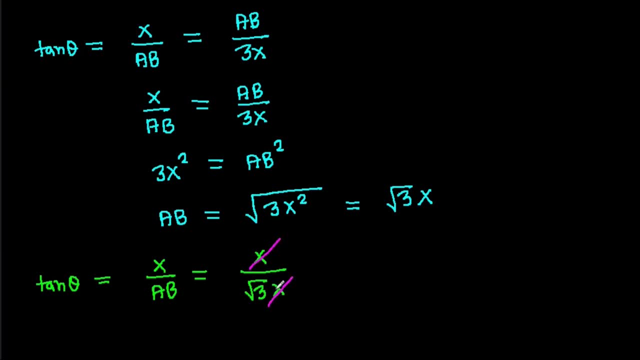 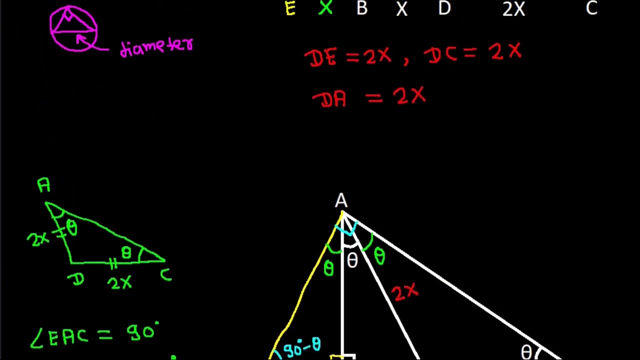 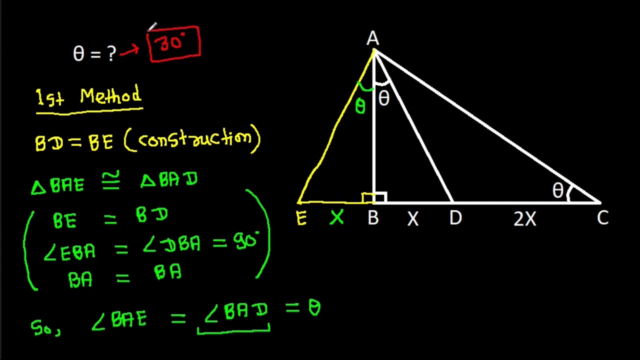 and x will get cancelled, so it is 1 over root 3 and tan theta is 1 over root 3. that means theta it will be 30 degree, So theta it is 30 degree, So theta it is 30 degree.